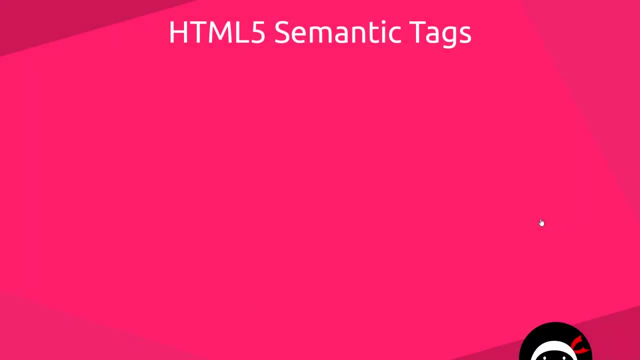 All right, then, gang. So we've seen quite a lot of different HTML tags in this course so far, but now I'd like to bombard you with some more, and they are the HTML5 semantic tags. So HTML as a language is always evolving, and there's always new elements that are being 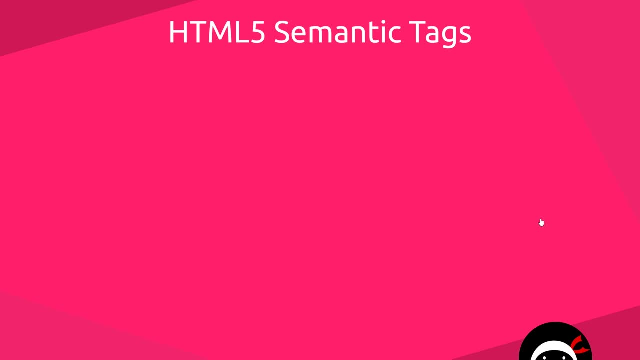 talked about or added to improve semantics and usability of websites. Now in the HTML5 specification there were several new tags that were shipped in in order to help us better structure our content properly and, I guess, more descriptively as well, so that now a browser can. 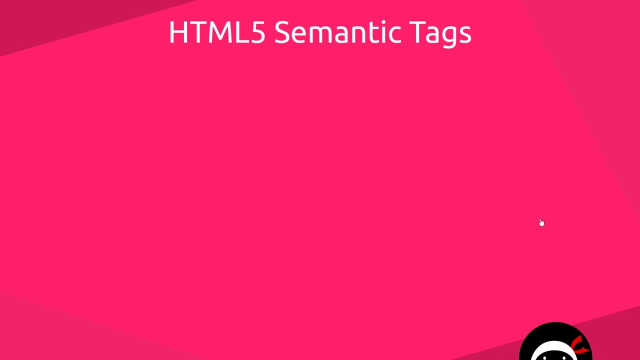 be in no doubt as to what our content is all about. For example, say, we put some content in a div tag, then the browser really has no idea what this content inside it really is. Could be an article, could be a biography, could be some quotes or some navigation links, etc. There's nothing. 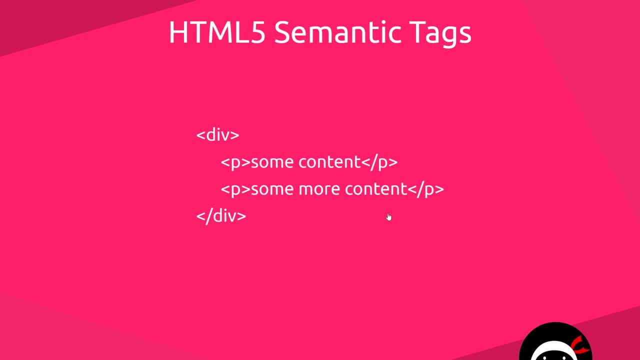 really here telling the browser what that content actually is? Now, HTML5 semantic tags aim to make our code better, but they don't really do that. So what we're going to do is we're going to make our code more meaningful and solve this problem. Well, it's not really a problem, but it. 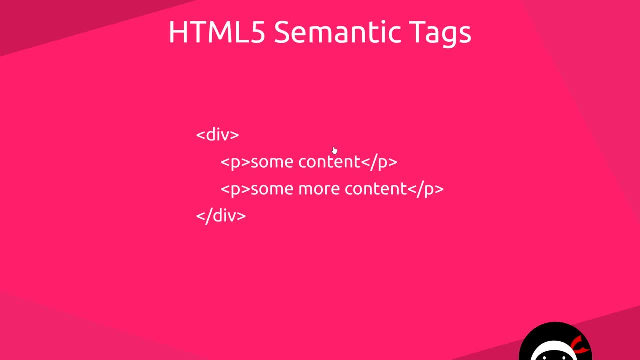 makes our code more descriptive. So now we could say instead: this is an article and use an article tag. This is an HTML5 semantic tag and it tells the browser a bit more about what this content is. It's a bit more descriptive. So let's have a look at some of the different tags, the different 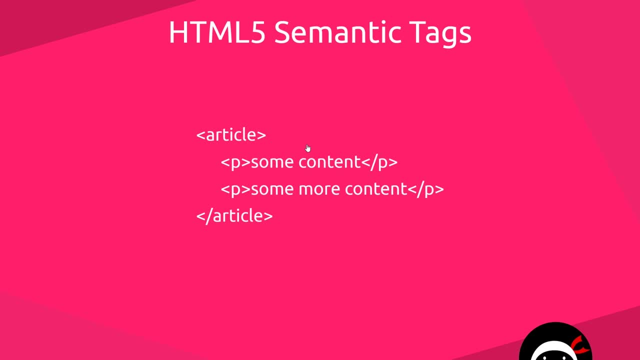 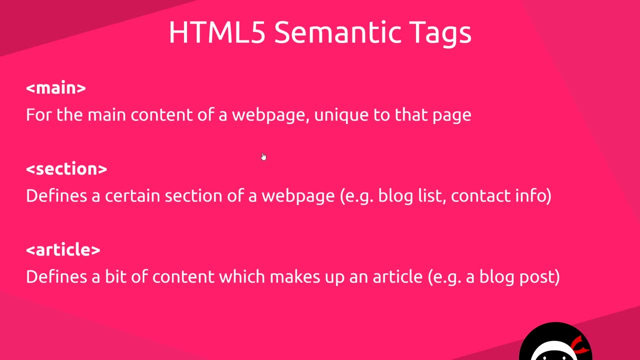 semantic tags that came along for the ride with HTML5. So first of all we have this main tag and that's for the main content. So let's have a look at some of the different tags, the different content of a web page, The bit that's unique to that web page as well, and it's not on other pages. 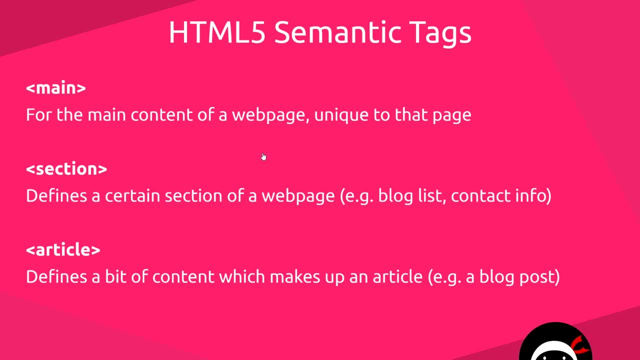 For example, it wouldn't include the navigation, because the navigation is on all web pages, but it might include the content, the main content of the homepage. So we have this main tag now. for that We also have a section tag and that defines a specific section of a web page And that could. 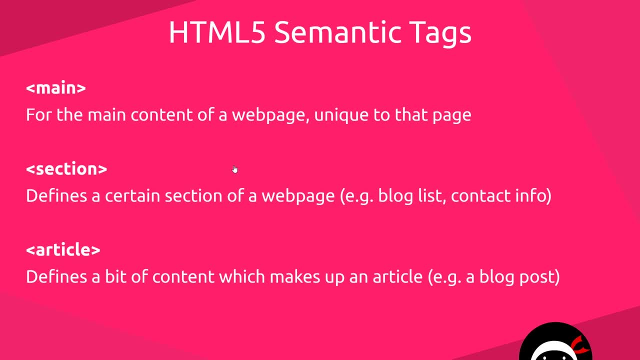 be a blog list or contact information or something else, And we could have several different sections on a web page. So we're saying, let's have a look at this, So, let's have a look at this. So we're saying to the browser: look, this is a unique section and it's kind of sectioned off. 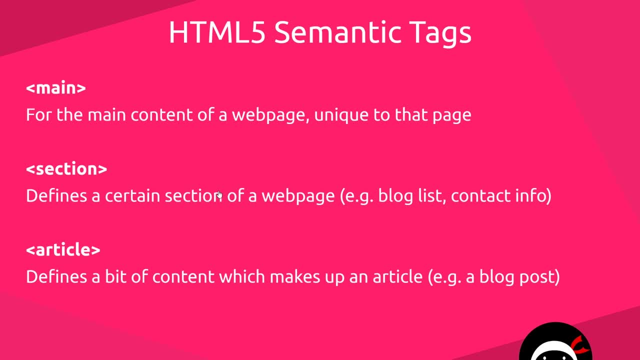 from everything else. It's got its own meaning. inside this tag. We also have an article tag, which I just showed you, And that's going to define a bit of content which makes up some kind of article. That could be a blog post, or it could be a news post or something else like that. 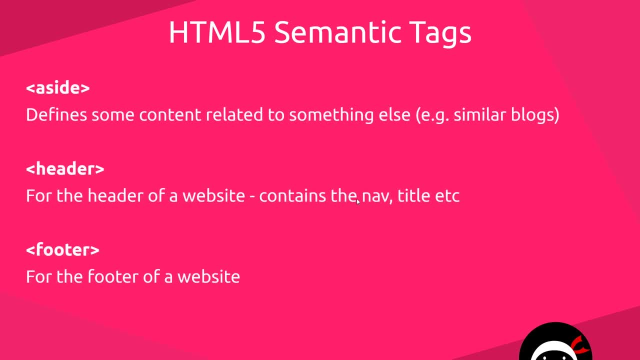 We also have an aside and that's going to define some content that's related to something else. For example, inside an article at the bottom, we could have a little section that is for similar blogs, And that could be an aside because it's still to do with the article. 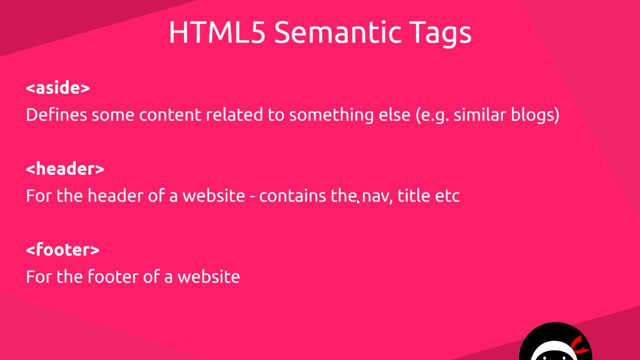 It's related to it, but it's not exactly part of the article. It's an aside, So we'd have those in an aside tag. We also have a header and that's for the header of a website. things that could be. 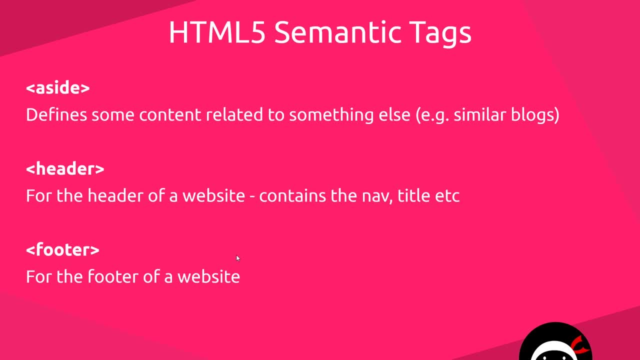 on every page. It could be the title, the logo, the navigation, etc. And we also have a footer and that's basically the footer. It speaks for itself. You could have contact information in it or a copyright notice, that kind of thing, And that's going to define some content that's related. 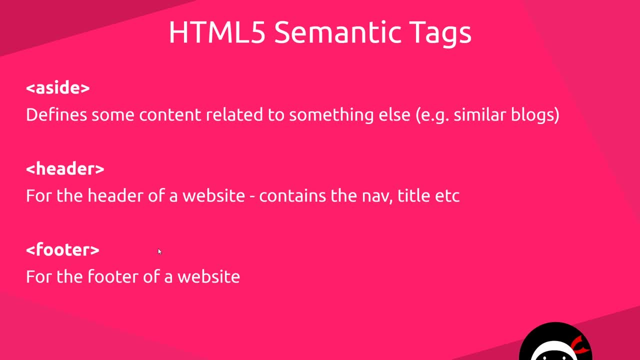 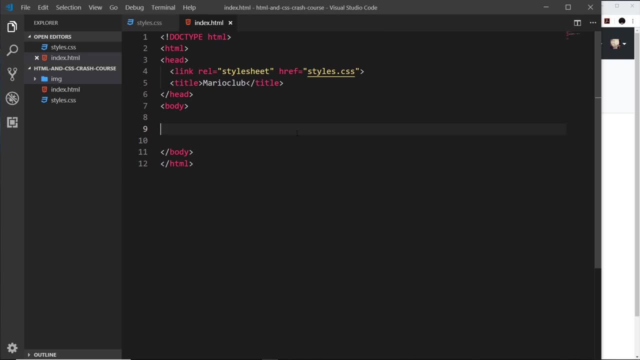 There's also more, which I will show you as well, but let's dive into the code now and start practicing with some of these tags. So then, my friends, for the rest of this video, what I'd like to do now is flesh out all the HTML for that mini project I showed you right back in the first video. 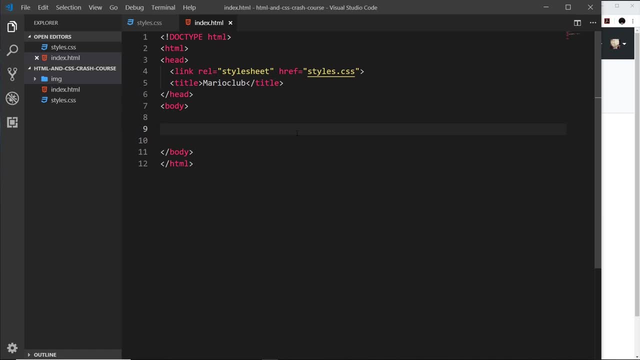 of this series for the Mario Club webpage. So to do this, I'm going to be using a mix of HTML5 semantic elements, which we've just talked about, and also some other tags that we've seen in the past. So before I start, you're going to notice that I've got this indexhtml file very blank at the 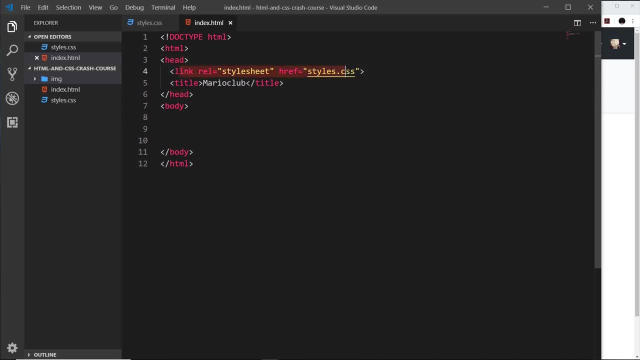 minute. I've just got a head up here and that links to a style sheet which is over here and there's nothing in there at the minute, so a blank style sheet. Then we have a title which says Mario Club. 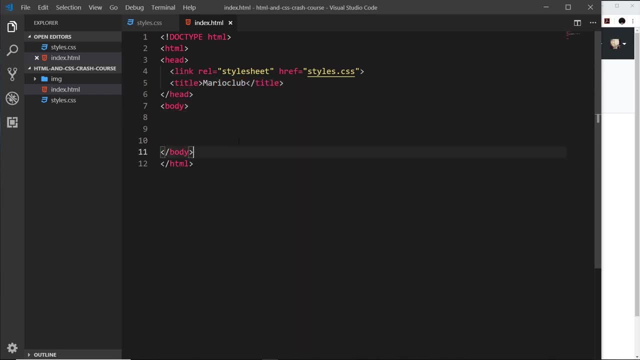 then a body as well. Now also, I'm going to be using several different images in this project as well. Now I've already added those over here on the left. I did that by going to new folder and calling it IMG for image. 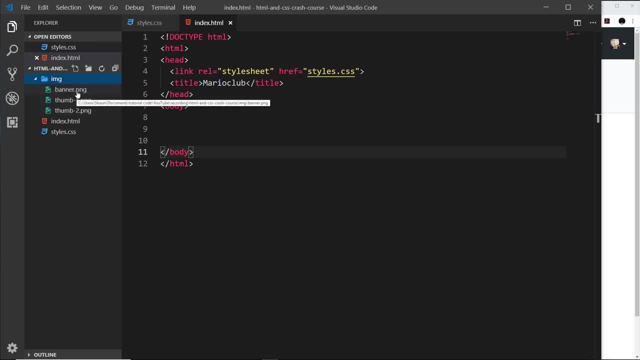 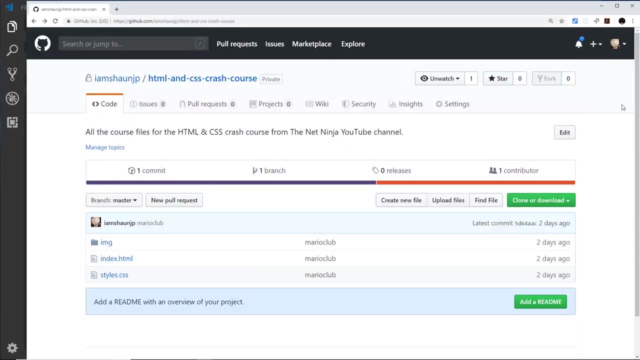 And then just drop it in the images that I wanted. Now I'm going to supply all of these images for you and you can find them on my GitHub repository, So I'm going to leave the link to that down below. It's going to show this page and you can either clone or download. So download the whole zip file for the entire project, which includes the image folder, the finished index file and the finished styles, Or you could just go into the image folder and each one of these files and right click and save as if you prefer. 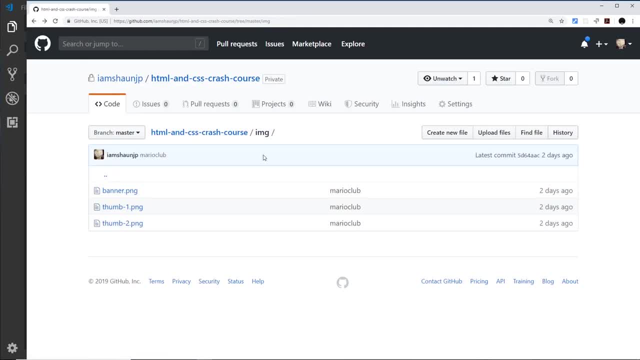 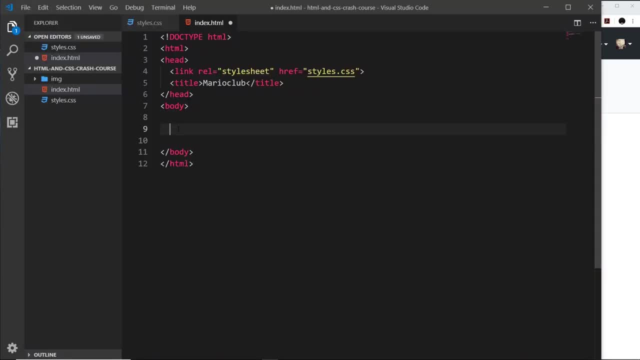 So that's the images. Now let's crack on with the HTML for this project. So then, the first thing I'm going to do inside the body is a header tag- Remember, this was one of those HTML5 semantic elements we just talked about- and the header is meant to contain things like the navigation or the site title, those kind of things. So, inside the header, all I'm going to do is an H1, and this is going to be the site title and it's going to be called Mario Club. 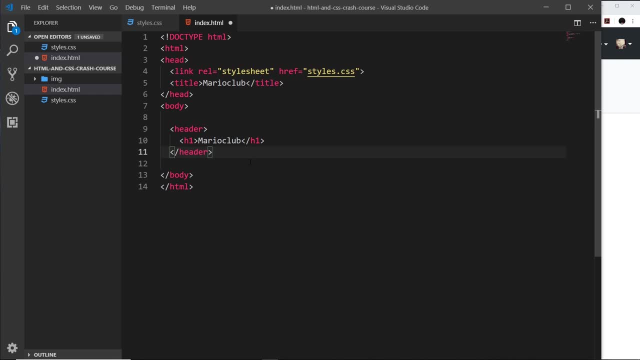 Okay, so that's the header all done. Very complex. Now next I'm going to do a section tag and this section is going to be for the banner. So what I'm going to do also is give this a class of banner, because we'll use that class later on to style this in the CSS. 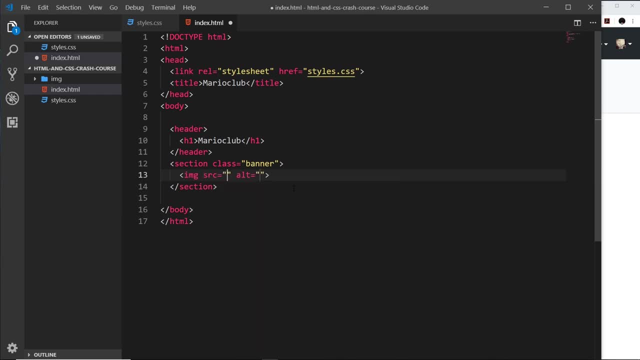 Now, inside that, what I'm going to do is first of all an image, and the source is going to be the banner. So it's inside the image folder, then it's bannerpng. So I'll say image For the image folder and then bannerpng. The alt is just going to be something like: Mario Club Welcome Banner. 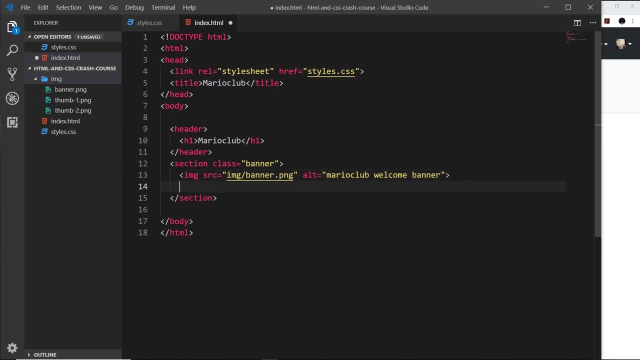 Okay, so after the image, I also want a little div tag, and this div is going to basically be a little welcome message on the banner itself. So what I'll do is again give this a class and that is going to be equal to welcome, because again, we'll use this class as a hook later on. 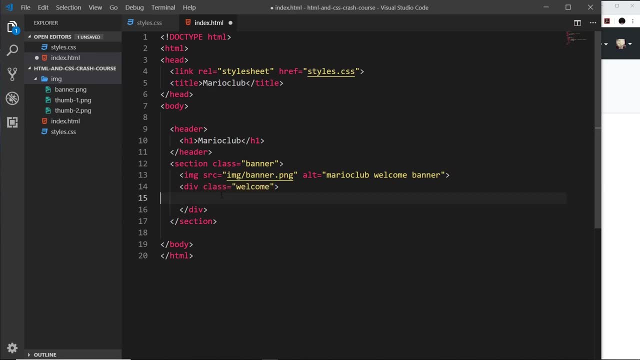 when we want to style it from the stylescss. So inside the div I'm just going to do an h2, and that is going to say welcome to, and then I'm going to do a br tag because I want to go to the next line and I'm going to do a span tag as well because we're going to hook into this. 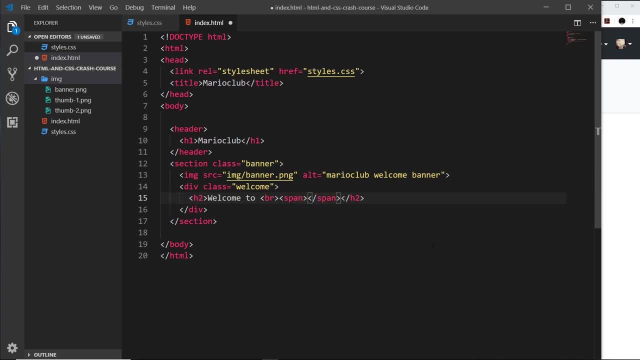 and style this word inside this span tag differently later on, and it's going to be Mario Club. Okay, so now we have this section done, That is going to be the top Banner and inside that we just have an image and then a little section, this div, right here for the welcome message. 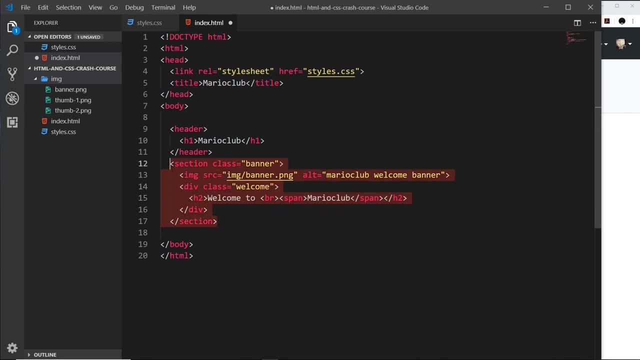 and that's going to sit on top of the image later on. So all of that is inside this section, So we're using our semantic tags quite well, so far, Okay. so the next bit is going to be a little navigation that lives under the banner. 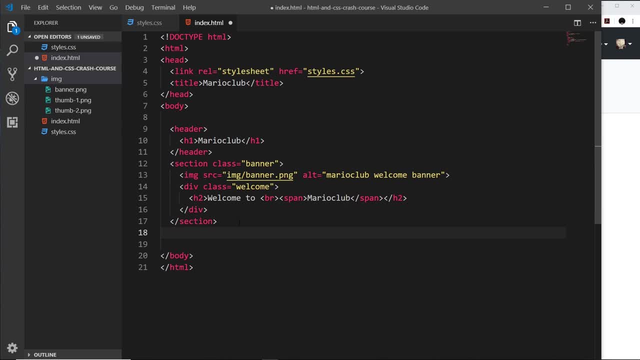 So to do that again, I'm going to use an HTML5 semantic tag. We've not seen this one yet, but it's called nav and I'm also going to give this a class, because I might want to use this class later on from the CSS, and that is going to be main-nav. 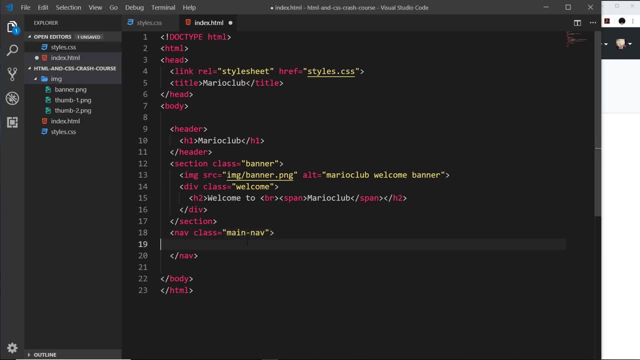 And we can have hyphens in classes. by the way, That's absolutely fine. And inside this nav, I'm going to do a ul and I'm going to do a series of list items, So each list item is going to contain a link, basically. 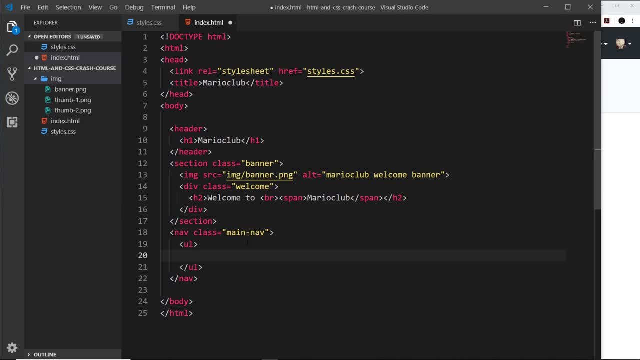 And this is a common thing that I do when I'm creating navigations- I often put them inside li tags, So I'm going to do the first one and inside there, an anchor tag. It doesn't matter, It doesn't matter. 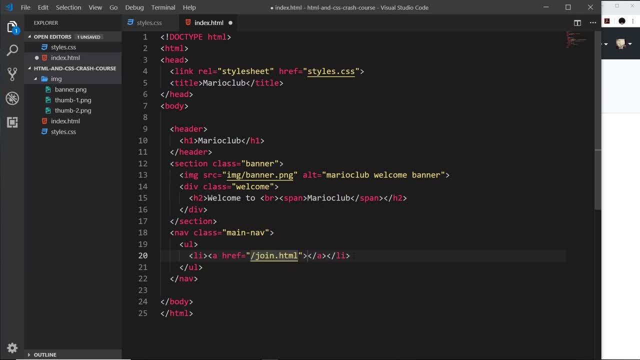 It doesn't matter where it's going to go at the minute, because we're not going to create all of these pages. So I'll just say joinhtml, and then the link text is going to be something like join the club. Now again, I'm going to give this a class, because I'm going to style this link differently from the rest. 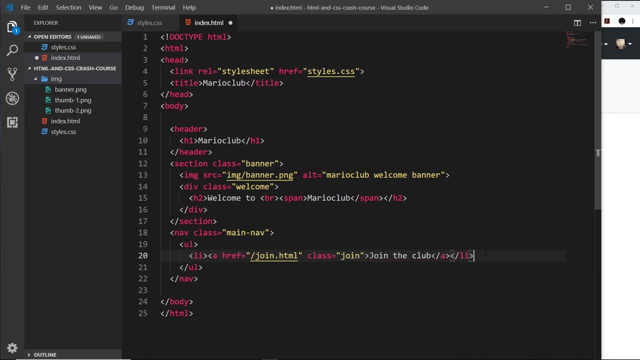 and I'll need this class later on to do that. Okay, so the next li tag inside is also going to have an a tag. The href this time is going to be forward slash newshtml And then inside we'll have the text be latest. 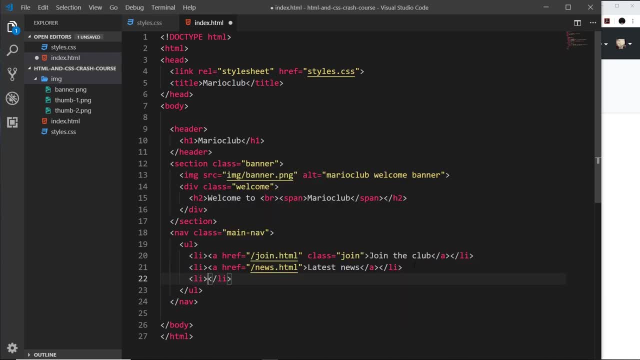 News, And then down below we'll do another li tag, another anchor tag. The href can be forward slash- gameshtml. And then inside the text can be new games, All right. And then finally one more, And inside that we'll do another anchor tag: forward slash contacthtml. 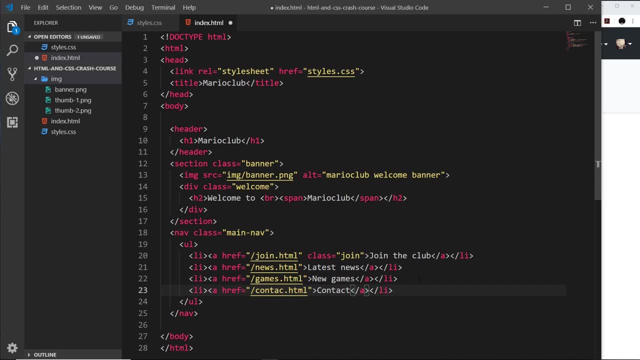 And then inside that we'll just say contact. Okay, so now we've created our navigation And that again is inside And html5 semantic element nav, intended for this kind of thing. Now the browser knows that this is a navigation. 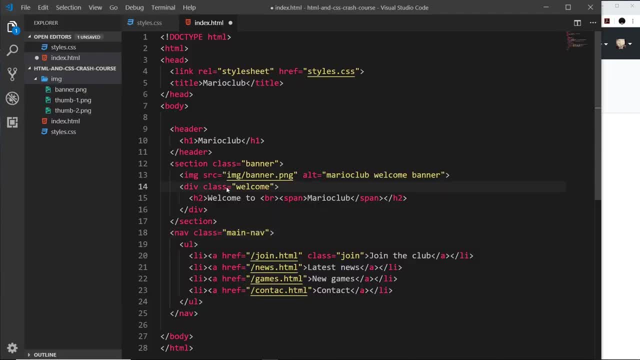 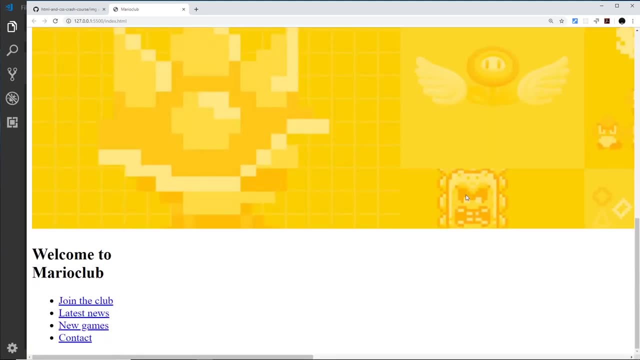 Now what I'm going to do is preview this in the browser, So I'm going to right click and open with live server, just so we can see what it looks like. so far, A complete mess. But there we go. That's the html, not the css yet. 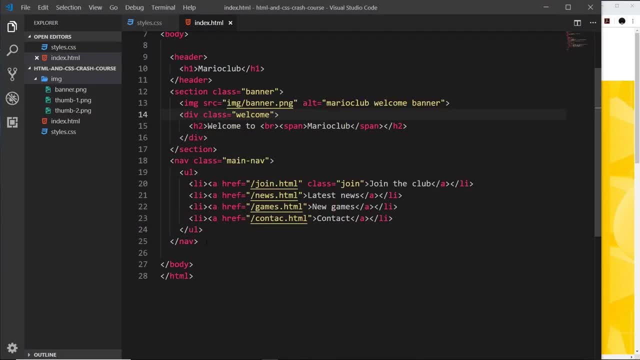 So hopefully, later on it will start to look better. But anyway, let's carry on now with this template. So, after the nav, we're going to have the main section. We're going to have the main section of the website, the content of the homepage. 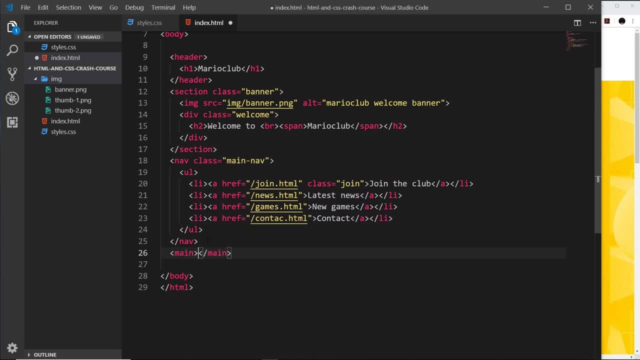 So remember I said we could use the main tag to do that. That's going to be the main content on this webpage, unique to this webpage. Now, inside this main tag, first of all, I'm going to have a little article at the top about the website. 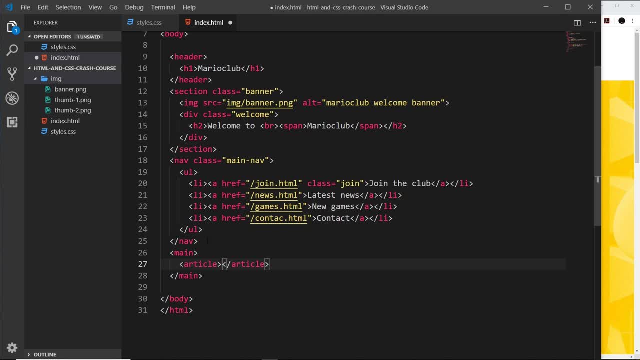 So that sounds like a good opportunity to do an article tag. So inside the article we'll do a title, first of all h2. And then I'll say: there it's a me, Mario, All right. And then underneath that I'm going to do a paragraph tag. 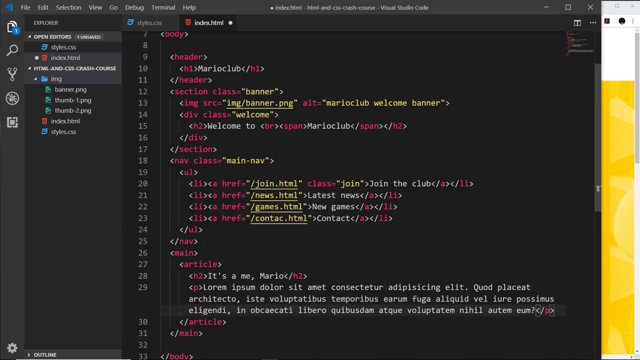 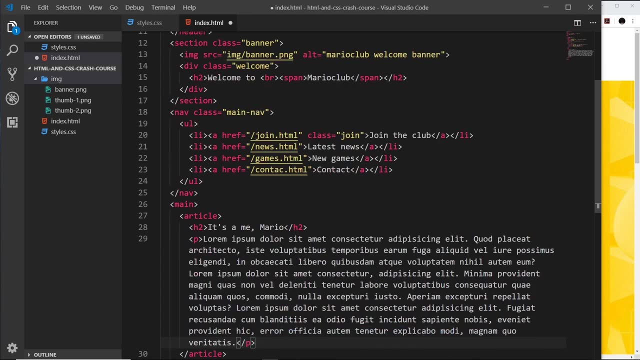 And inside this paragraph tag, just a load of lorem ipsum. So let me do that a couple of times Lorem again, And I'll do it one more time Lorem, like so Okay, so we've got some dummy text now at the top inside this article tag. 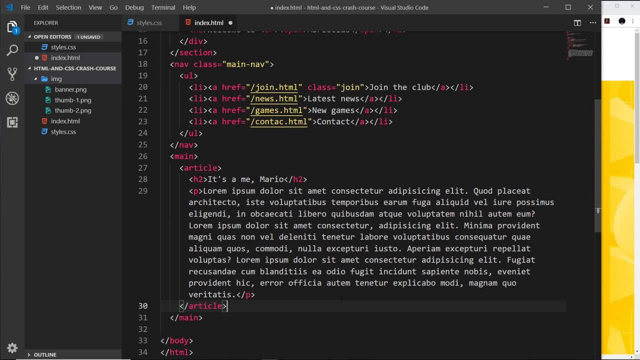 Then, after the article, I'm going to show a couple of different images. Again, I'm going to put these in a ul and some li tags. So each image is going to be in an li tag And typically, again, when I'm showing a list of stuff, I typically put them inside li tags. 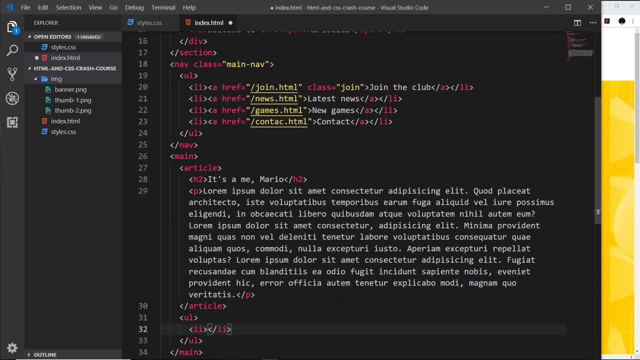 It doesn't have to be a logical list like a shopping list. if you want to use li tags, It can just be a list of images or a list of icons or, you know, even things like this: a list of links. 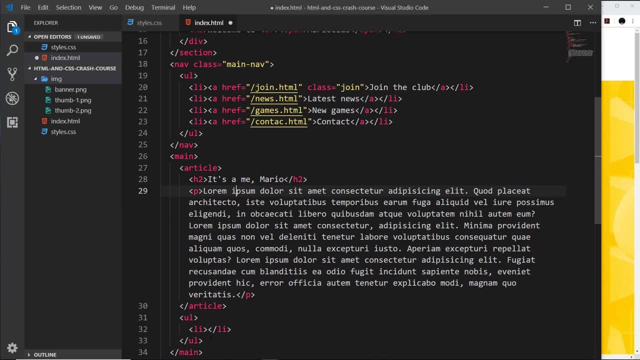 So I'm going to place the first image inside here And in fact, what I'll do is give this ul a class equal to images Again, so we can hook into this later and create a selector so we can target this. 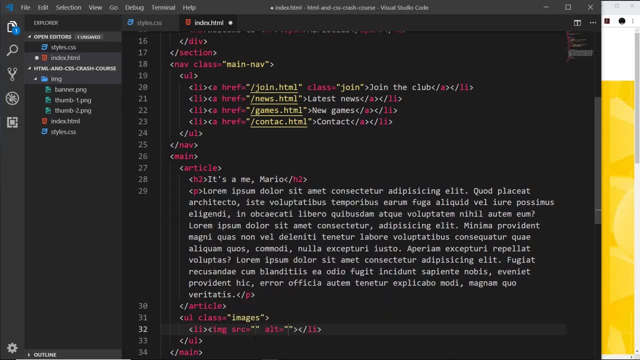 So inside this first one we'll do an image tag And the source, remember, has got to go to one of these, So it's inside the image folder forward slash. thumb hyphen one dot png. Okay, the ults can just be something like: Mario, thumb one. 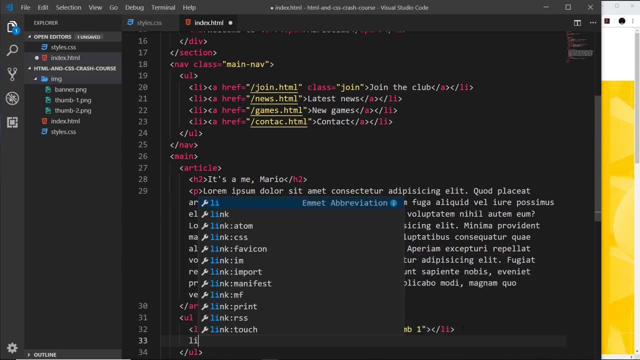 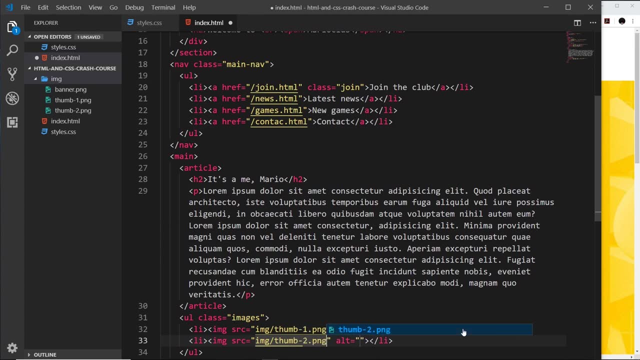 Very descriptive. Okay, so the next one inside an li tag again is going to be another image, And this time the source is going to be image forward slash. thumb hyphen two dot png. Okay, Okay, Okay, Okay. 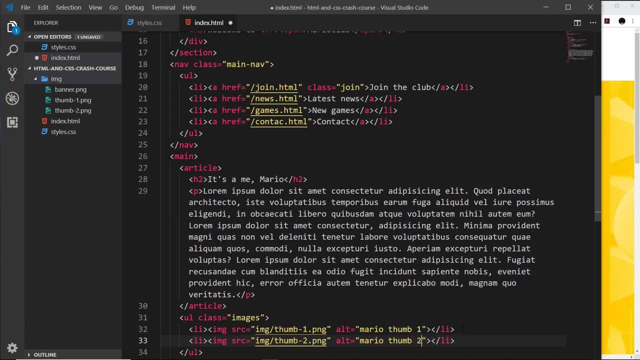 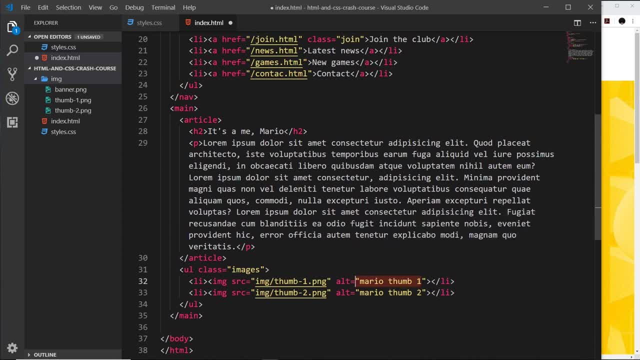 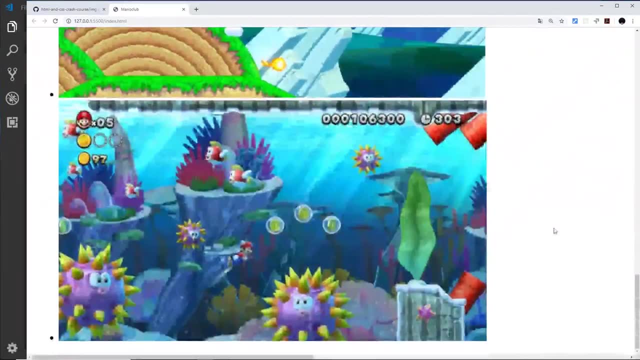 I can't think of anything off the top of my head, So that's why I'm doing these lame ones. Anyway, now we have these two images I'm going to save and see if these look okay. so far, No, they don't. 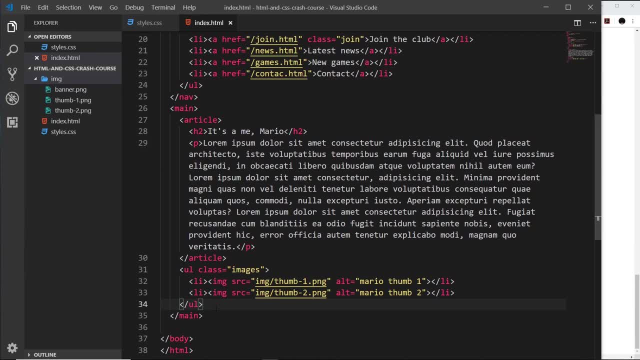 But, again, we'll make this look better later on. Okay, So, after those images, what do we want then? Well, that's going to be after the main content, because it's going to start to be the footer now. Okay. 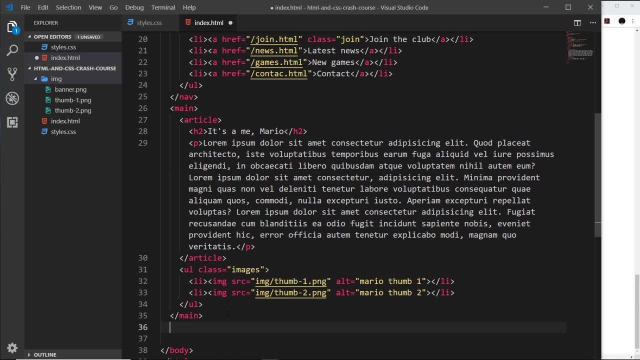 Okay, Okay, Okay. Okay thing i want is a little section just above the footer which is going to be a form for a user to join the mailing list. so i'll do a new section for this and this is going to have a class of join. 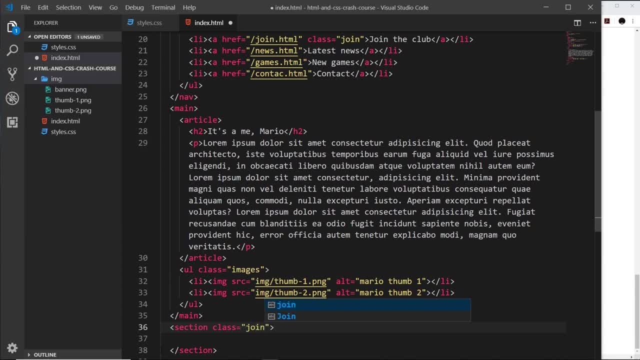 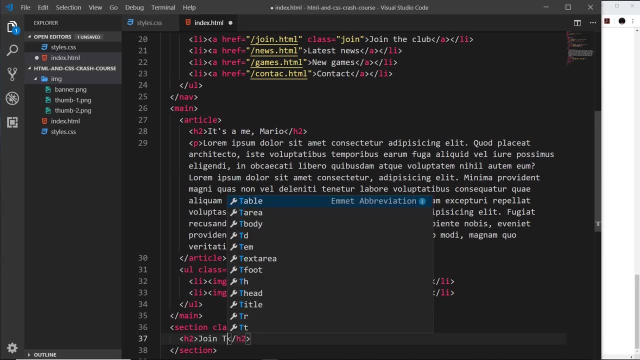 so later on i can target this section with a selector looking for the class of join, and then i can style this differently. so we'll do an h2 inside and we'll say join today- exclamation mark, and then we'll do a paragraph tag. we'll just do some lorem ipsum in there. we. 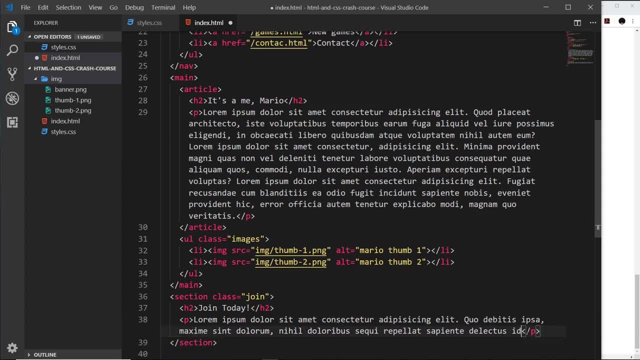 don't need all of that. so let's just delete a bit of it, just go back to the id and then after that we need to do our form, so let's do that form tag. we don't need the action because we're not going to be sending this to a server. this is just the front end. we're doing at the minute the html and 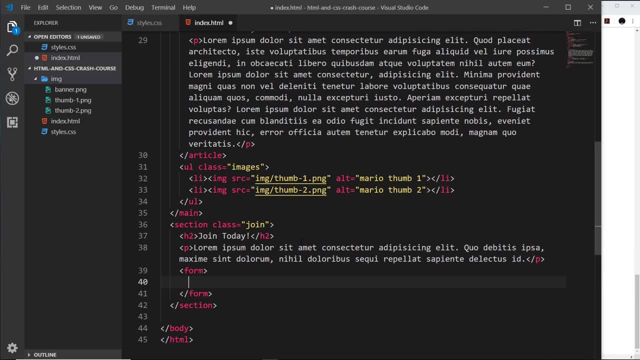 the css, but inside the form we need an input field for the user's email. so we'll say input and then the type is going to be email. now i'm also going to give this a name, property or attribute rather, and that is going to be email, and i'm also going to give this a placeholder. so we're using knows.